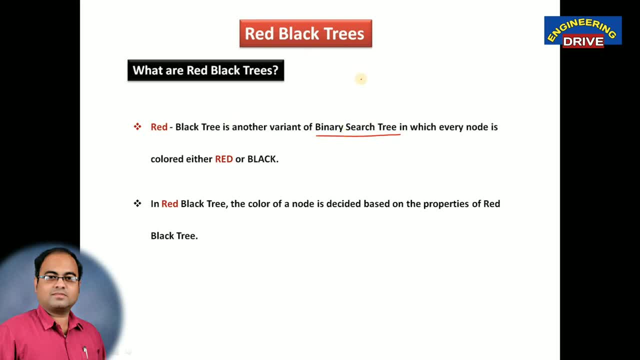 That you need to remember. That is the condition of a binary tree. Okay, left child value must be smaller than the parent node. Right child value must be greater than the parent node. If this condition is satisfied, then we can term this tree as a binary search tree. 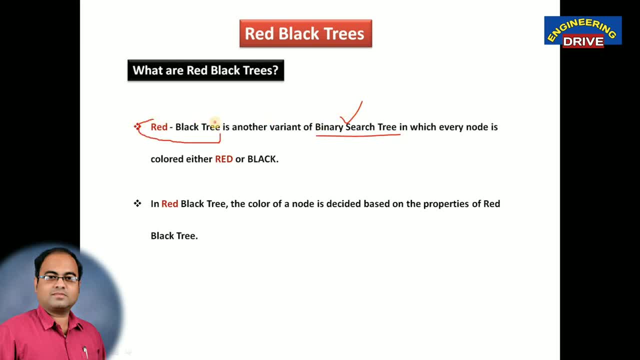 So the same condition is applicable for red black tree also. Okay, that you need to remember. And one more new thing that is added: in the red black trees, as the name suggests, Every node is going to be colored either red or black. Okay, this is very, very important. 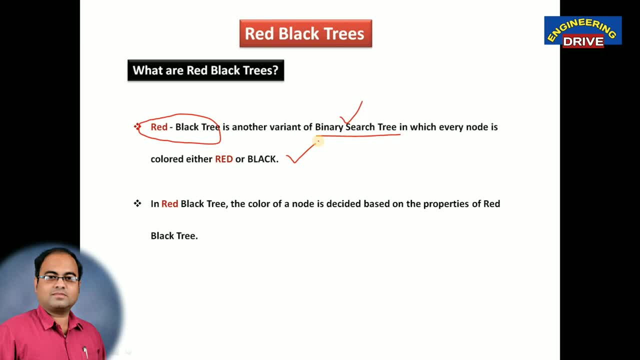 Here. you are not going to keep the nodes without any color. It is mandatory for you to either fill the node with a red color or black color. Now the question that will come in our mind is, sir, which node should be selected as red and which node should be selected as black? 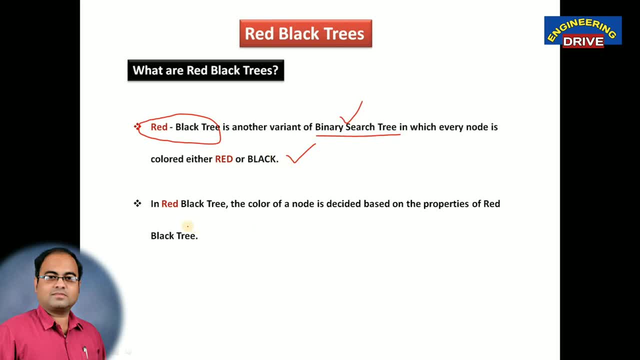 Then I am going to speak out in my next slides. Okay, now you can see here the second point. In red black tree, the color of a node is decided based on the properties of red black tree. Okay, this is very, very important. 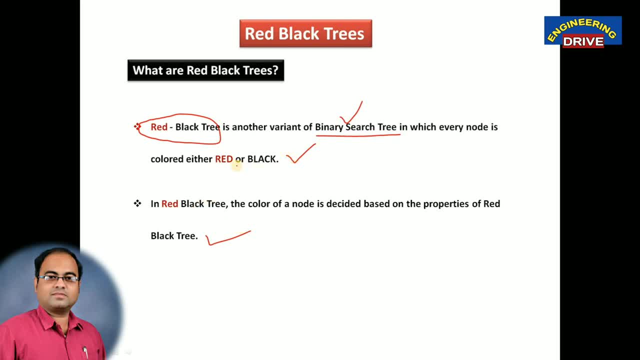 Now the doubt that was there in the previous point, sir, how to color the node as red and when to color the node as black. sir, So in red black tree, the color of a node is decided on based on what? Based on properties? based on properties of red black tree. 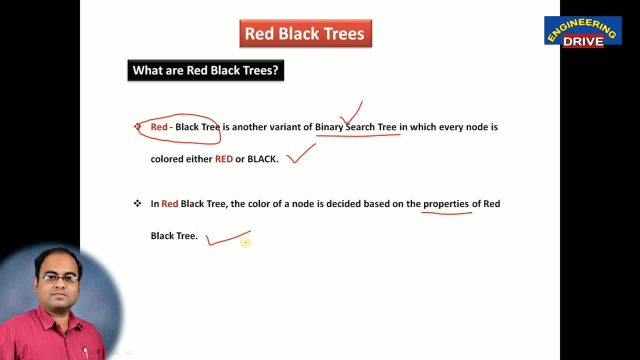 So you need to understand the properties of red black tree. Then you can able to decide which node should be colored as red or and which node should be colored as black. Okay, so to understand that concept, Let us start the properties of red black trees now. 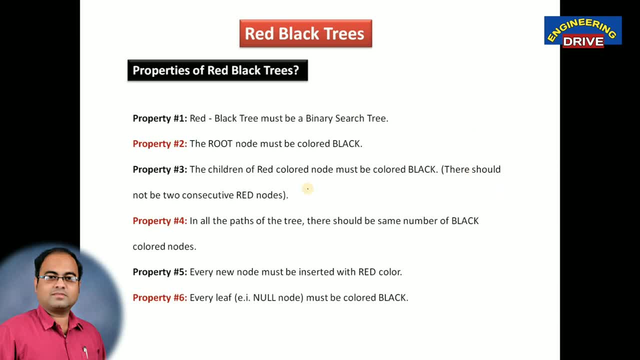 Okay now, properties of red black trees. So these are the six properties that each and every one of you should be able to understand and remember. based on that, we can able to create a red black tree. So, my dear students, let us, let us see one by one. 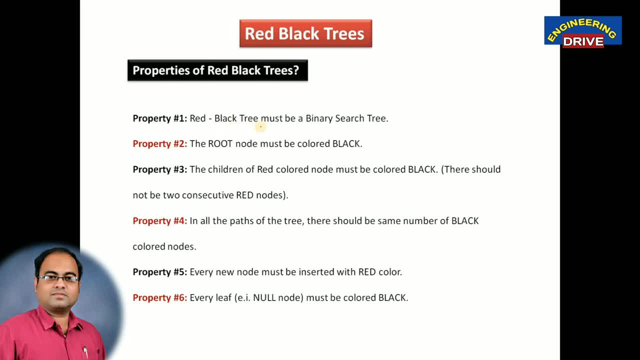 What are those six properties? Property number one, red black tree, must be a binary search tree. Okay, this is a mandatory condition because in the definition of red black tree itself It is clearly said that it is a type of binary search tree. 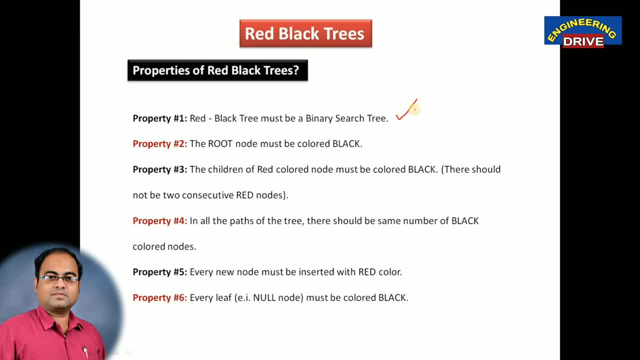 So, whatever the condition applicable for for binary search tree, the same condition is applicable for red black tree also. That is the first point. Now, while coming to the property number two, the root node must be colored black. So this is also a second very important property that will give a clear indication that the trees are red black tree. 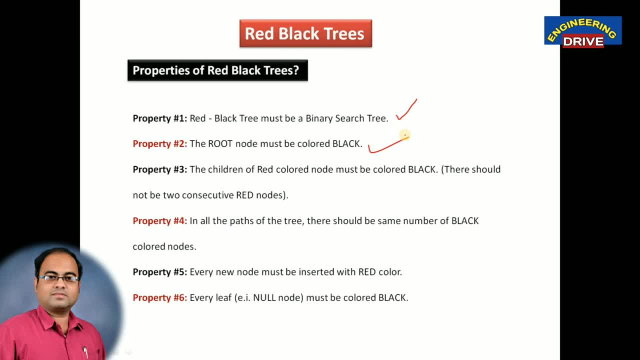 The root node must be colored black. So in the red Black tree if the node is in red color then we can't say that it is a red black tree, compulsory. The root node must be colored black. So you will remember this point. 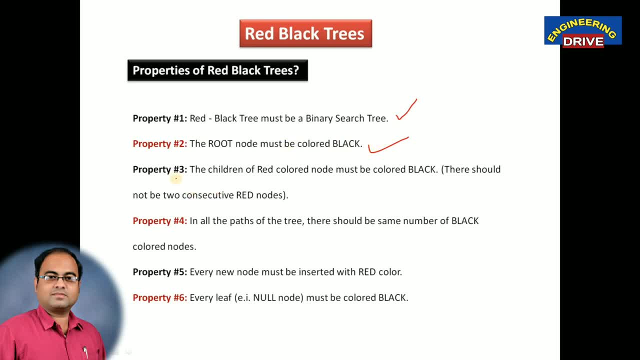 Always, the root node must be black in color And the property number three, the children of red color node, must be colored black. Now see here the children of red color node. there are red color nodes, their children's must be colored black. 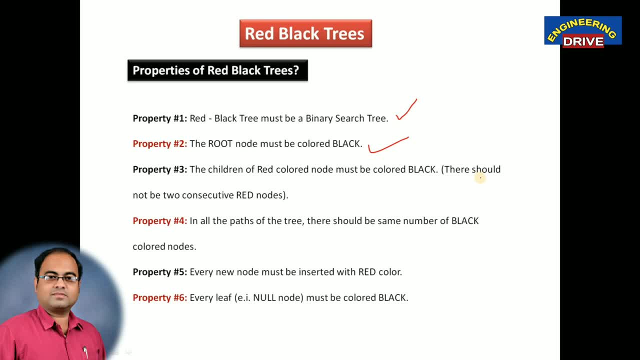 This is also an important point. Okay, And indirectly it is saying that there should not be two consecutive Two red nodes, which means, if the children's of red color nodes must be black indicates you will get first one red color node and next you will get one black color node, which means there should not be two consecutive red nodes. 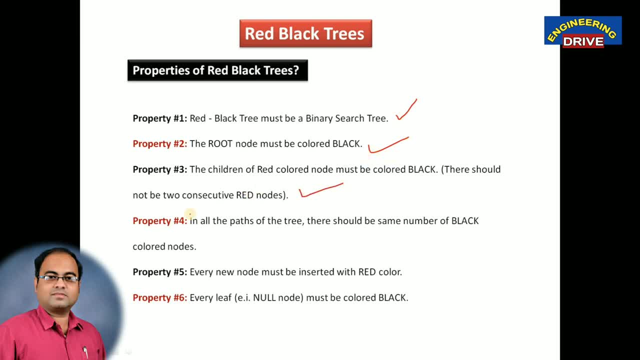 This point is also clear. So these are the three important properties And while coming to the property number four, in all the parts of the tree there should be same number of black colored nodes, So when you are traveling the path of a tree, always there should be equal number. 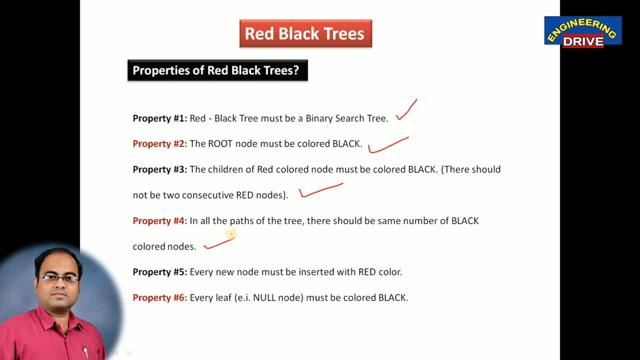 Okay, Black nodes that should be available in the red black trees. Okay, This is also a very, very crucial point. Okay, Next, property number five: every new node must be inserted with red color. So the new node which you are going to insert in the red black tree, it must be in red color. and the law. and the last property, property number six- every leaf or the null node must be colored black. 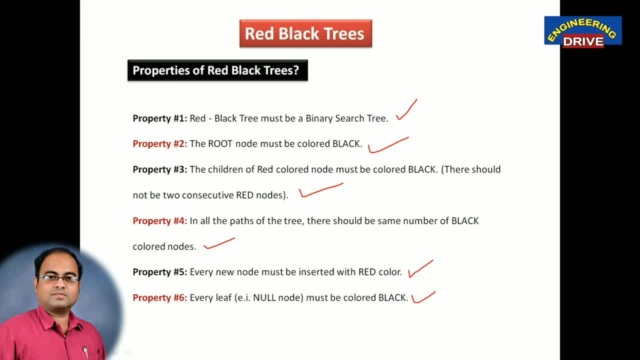 For example, let us say you want to specify the leaf nodes, which are null. So in which color You are going to use at the time you are going to make use of the black color. Okay, So this is the property number six. 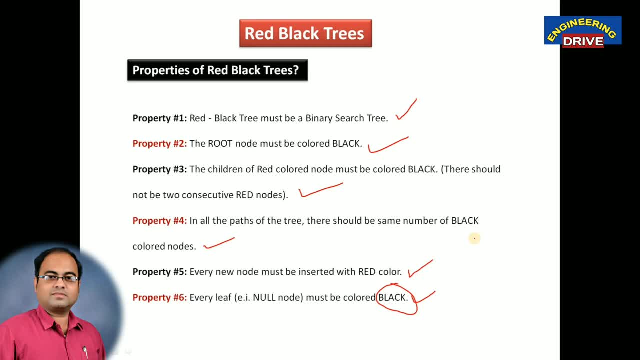 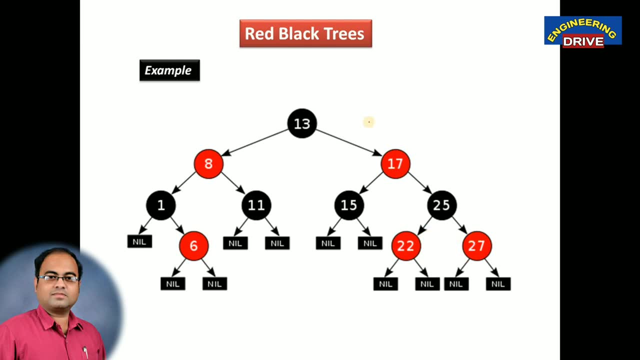 So, based on these properties, we are going to find out whether the tree is a red black tree or not. Okay, So, my dear students, let us take one small example now. So, whatever the properties I have discussed here, that's all those properties applied to this tree. 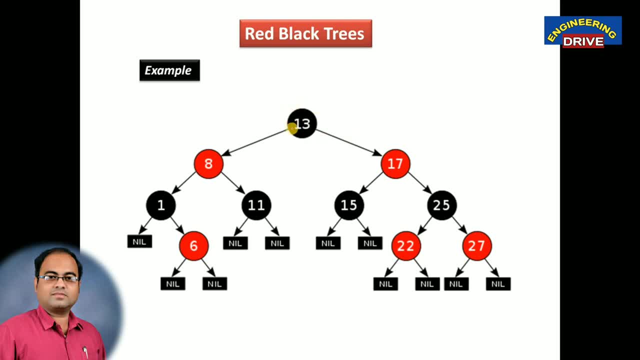 See here the root node we have taken, as in black color, and whether it satisfies binary search tree property. Let us see left node value. This is the left node value and this is the right node value. Left child value is smaller than the root node. 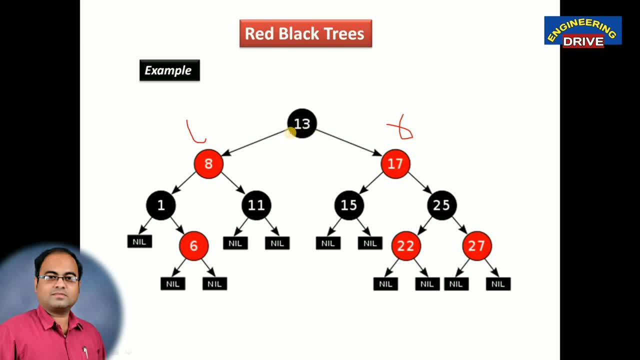 Right child value is greater than the root node. So of course it is a type of binary search tree. So red- black tree must be a binary search tree. that condition satisfied, The root node must be in black color. Okay, And there should not be two same consecutive color nodes or red nodes. 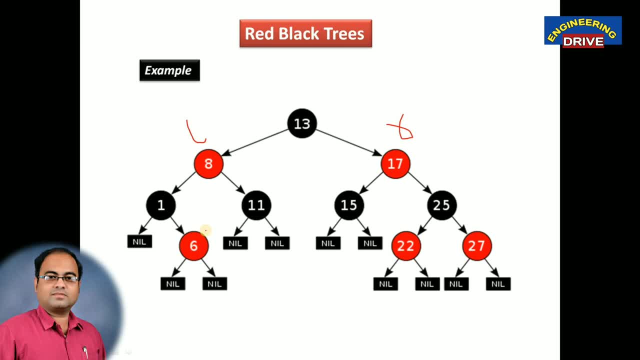 We can see here one black, one red, again one black, one red. This condition also satisfied. And I told one more condition: that if you are specifying the leaf nodes as nil or null nodes- both are we can use the terms nil or null- then compulsory, those nodes must be in black color. 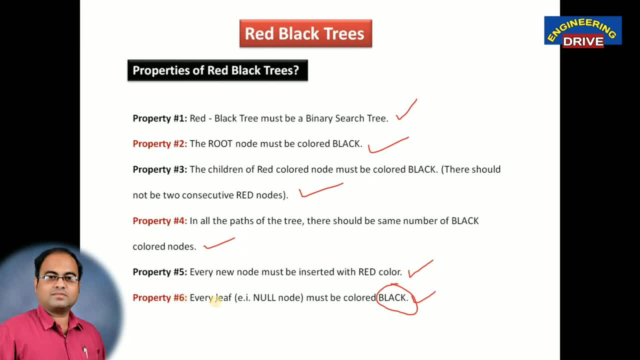 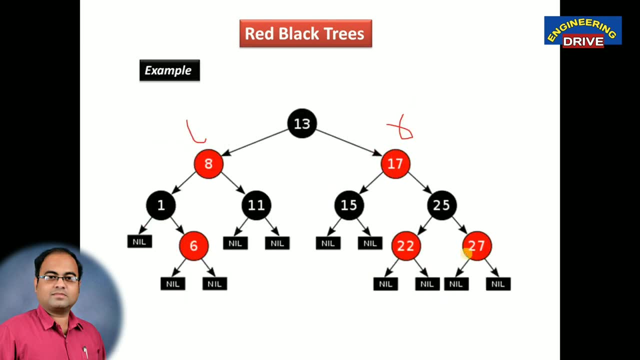 You can see here. So last property null node or the nil node must be colored black. Okay, So that's what we have used here. So the last leaf node. they are all termed as in black color Because they are the null or nil nodes. 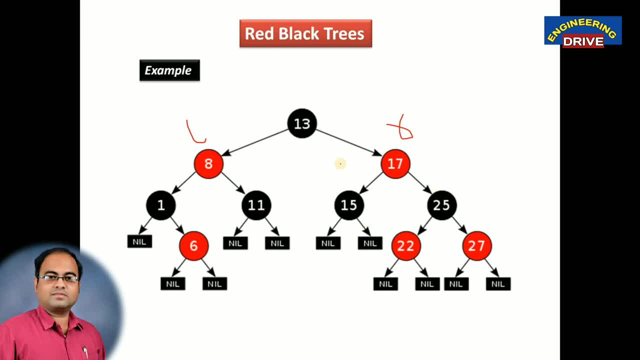 So if we, if all those six properties, are satisfied, then we can say that this is an example of a perfect example of a red black tree. Hopefully the point has been clear to you. So don't use red color If let's say, let us say, red color is available at the root node and it is not a red black tree. 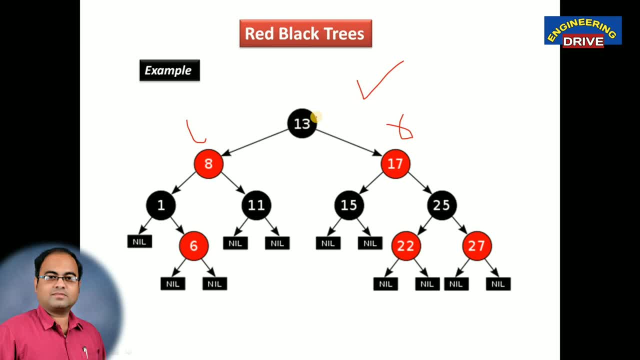 So you may get this type of bits in the multiple choice options also in the exams. So, my dear students, you carefully remember the main Concept of red black trees is color itself. When red color will come, when black color will come, can the tree will have two consecutive same colors? 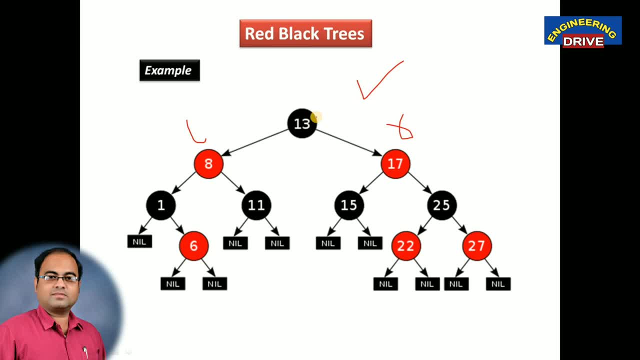 All these questions when you can understand, if you understand, the properties of red black trees? Okay, So with this we have completed all the concepts of binary trees. Five types of binary trees we have discussed. First number one, binary search tree. 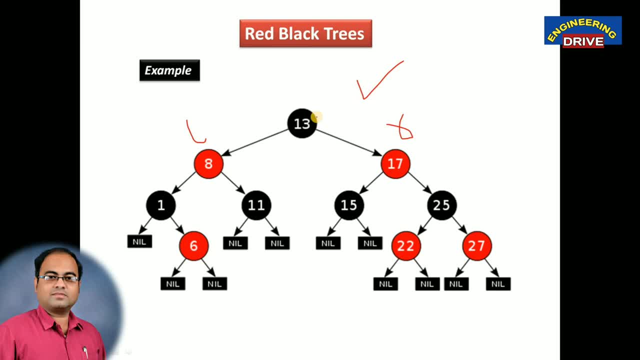 Number two, heap tree. Number three, avial tree. Number Four, D trees and the last one we have completed now, red black trees. So these are the five types of trees which are very, very important and compulsory. You will expect regularly one long answer, questions from this topic and even multiple choice questions in competitive exams.